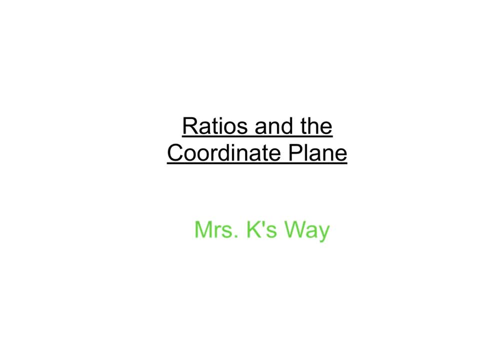 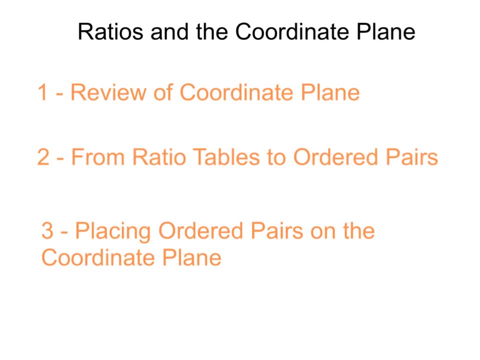 Howdy ho and hello there, neighbors. We are going to be doing a Mrs K's Way video about ratios and the coordinate plane. Of course, my videos usually talk about the three things that we are going to mention in the video. The first thing is review of the coordinate plane. What is it and what does it mean? 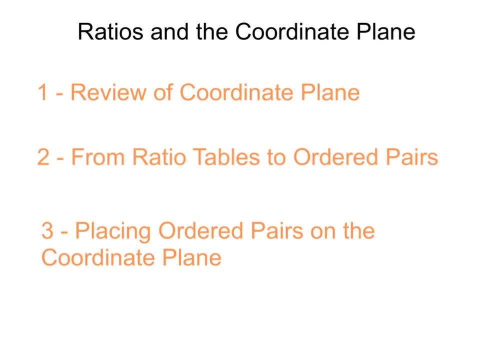 For the second thing, we're going to look at a ratio table we've been doing in class and seeing how to convert those to something called ordered pairs. And then, last but not least, we are going to place those ordered pairs on a coordinate plane. 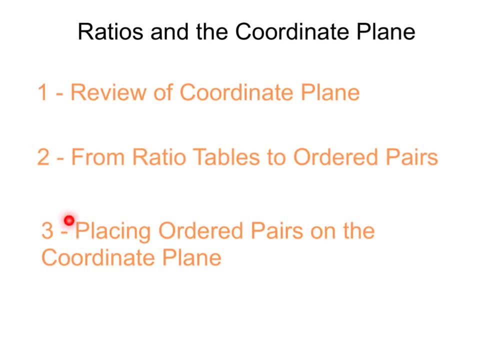 Kind of taking number two and number one and placing all together in step three. In today's video we are going to look at three different parts. We are going to do a very in-depth review of the coordinate plane. We're going to go over how to make ratio tables into ordered pairs. 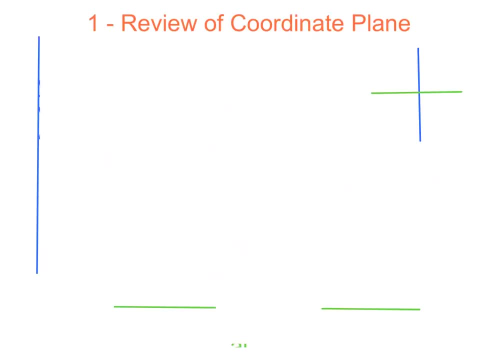 And then we're going to place those ordered pairs on the coordinate plane. So the first thing we want to remind ourselves is the coordinate. I have a small little coordinate plane over here in the corner And it's not labeled, but I just want to remind ourselves of our previous understanding of the four different quadrants. 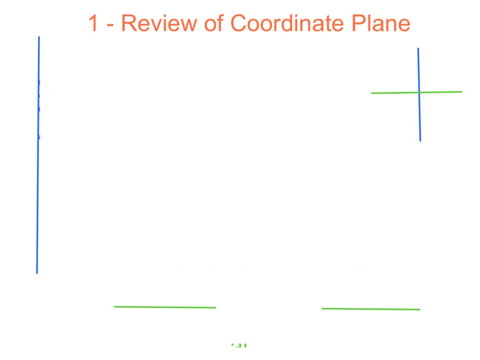 Since we have two lines that intersect, we have four different spaces and those are four different quadrants. We remember that we always start in the top right corner, since these are both our positive x and our positive y values. We have our second quadrant. third, 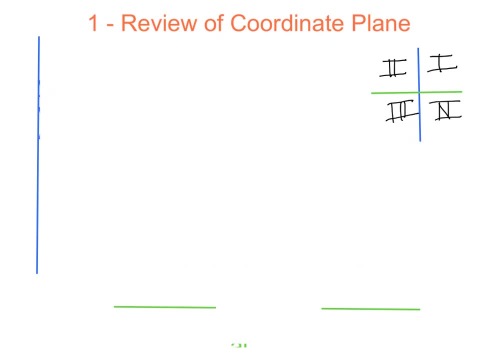 And we have our second quadrant, third And our fourth. Since we're using Roman numerals, it has a 1 and a v. We're going to talk about the first quadrant right here And let's look to see what one looks like a little larger. 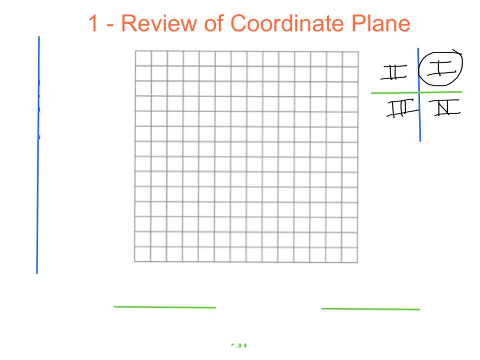 When we're labeling our first quadrant, we have two different parts to it. The first part that we have is this bottom line right down here, The bottom portion. We remind ourselves that this is called the x-axis. We also call it Our horizontal axis, which means that this axis goes from the left to the right or from side to side. 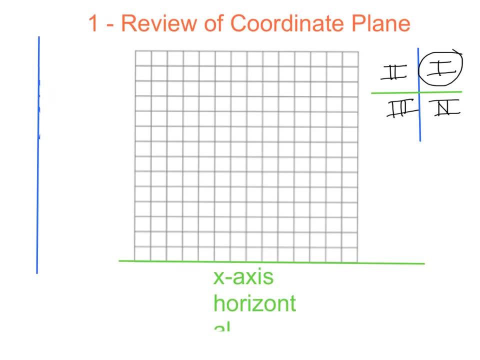 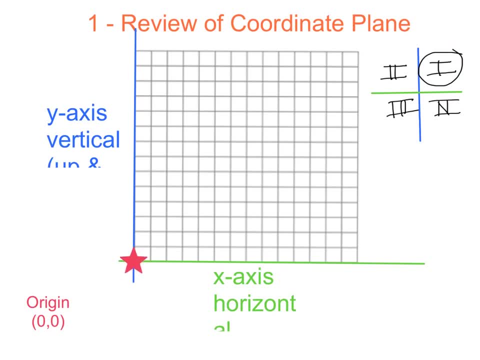 We call it the origin, And that's exactly where the two axes meet. That happens to be the exact coordinate every single time, which is going to be an x-coordinate of 0 and a y-coordinate of 0.. Next, we're going to be talking about how we can find other coordinates within the coordinate plane. 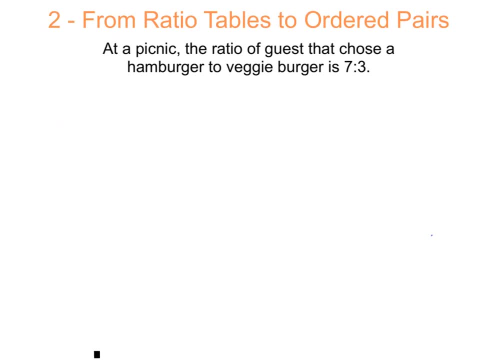 So, in order to find different coordinates or different points in our coordinate plane, let's look at an example here. At a picnic, the ratio of guests that choose a hamburger to veggie burger is a ratio of 7 to 3.. Now, when we're trying to figure out what this ratio is for, let's say, a larger amount of guests, 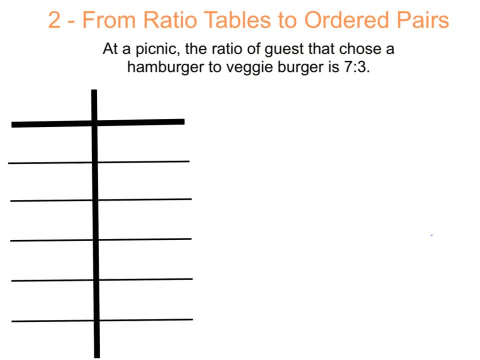 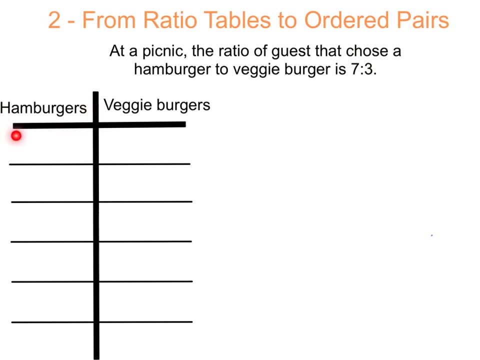 we can make a ratio table. What we want to do here is we want to be able to have our two different parts of our table represent our ratio here. Whoops, our ratio right here. So let's see how that looks. So first I'm going to put my hamburgers- since that's the first part of my ratio- on the left side of the table. 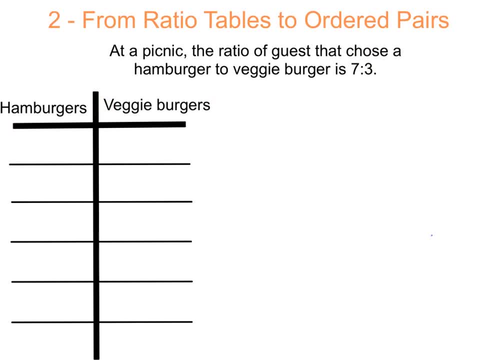 and I'm going to have veggie burgers on the right side of my table. Now, if I want to be able to fill in the table accordingly, I'm going to be using my ratio of 7 to 3.. So, if we fill out the table, it will look like this: 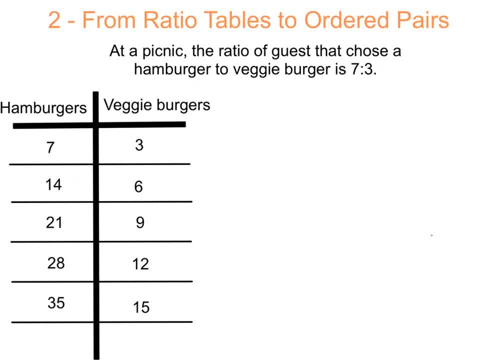 So my ratio table: if I have a ratio of 7 to 3, then I know that if I have two groups it would be 4 to 6, and we've been filling those out recently in class. Now, in order to now make these different numbers in our ratio table into ordered pairs: 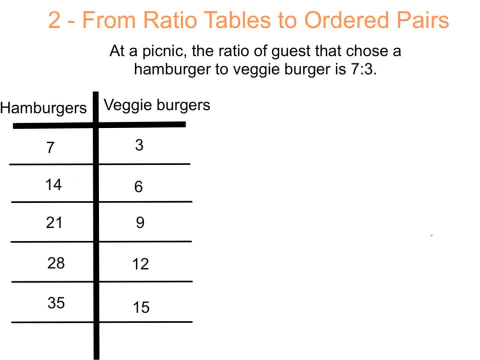 we're going to be looking at all of our hamburgers as our x-axis and our y is going to be veggie burgers, So I just color coordinated to help us, like we did with the last side, knowing that anything in green is going to be our x. 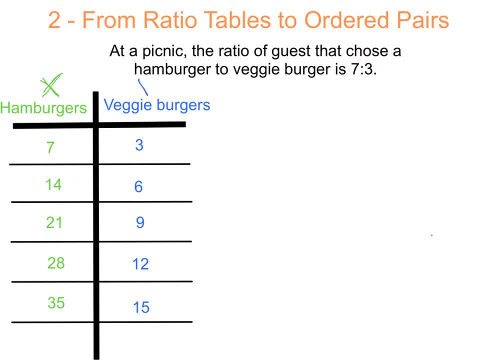 And anything in the blue is our y values. This also happens to be because the x values come first and the y values come second. How we know how to create the ordered pair is because the ordered pair are the coordinates of a point, written as x coordinate, y coordinate. 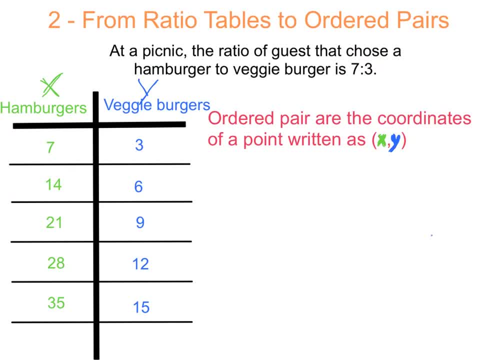 So each of these, we now have an x and a y coordinate. So if we wanted to try and make an ordered pair, for our first ratio we would have the ratio of 7 to 3, and our ordered pair would be 7 comma 3.. 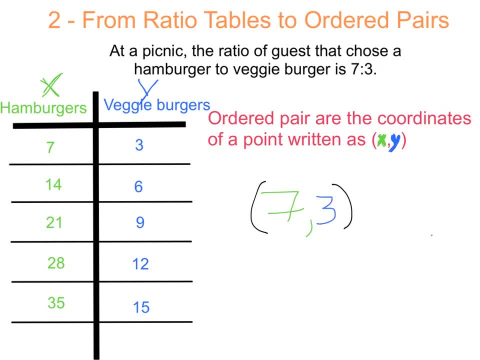 We want to put those around parentheses so that we know that they're points and we're not doing any operations with them. So let's see what the rest of the ordered pairs would look like. So our ratios would then turn into the coordinate pairs: 14,, 6,, 21,, 9,, 28,, 12,, 35,, 15,. 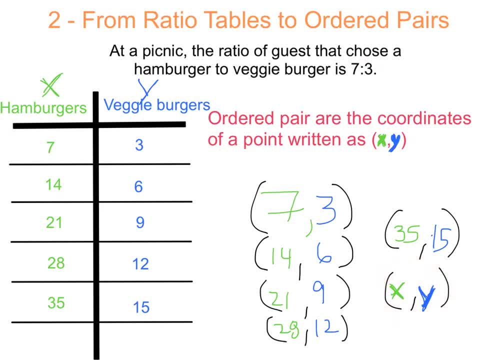 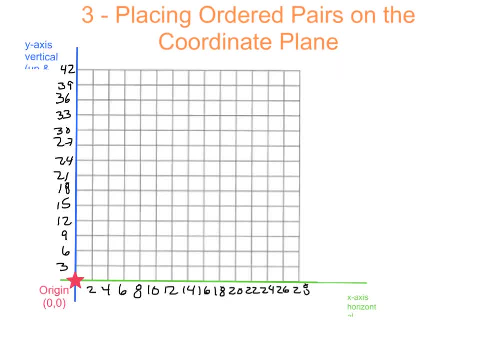 and any other future x and y coordinates that we would have. So that's what we have on our ratio table. Now that we have our ordered pairs, graphing them on a coordinate plane is a breeze. So let's first remind ourselves of our different ratios that we had on our ratios. 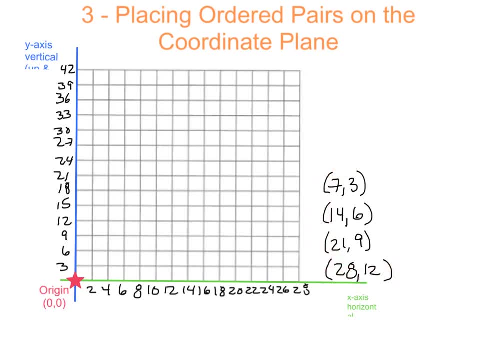 then we created a ratio table and then we created ordered pairs. We want to remind ourselves that the first one happens to be our x coordinates and our second part of our ordered pair is our y part of the coordinate. Now to be able to graph these on a coordinate. 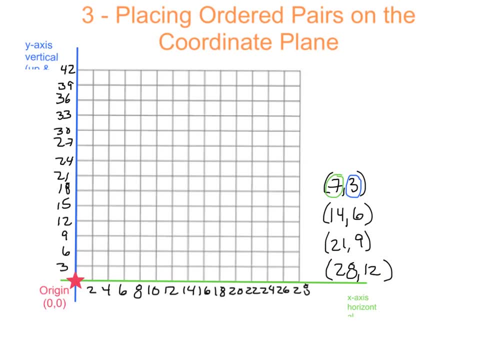 there's four simple steps. First step is: we start at the origin. So we want to find our origin 0, 0, and we're going to start here as our starting place. Second thing we're going to do is move in the x direction. 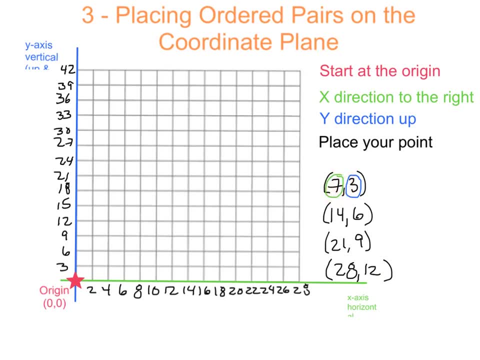 as many times as it tells us in our ratio or our ordered pair. So we start at 0,, 0, and we're going to move all the way to 7.. 2,, 4,, 6,, 7.. Then we're going to go up in the y direction as many times as it tells us in our ordered pair. 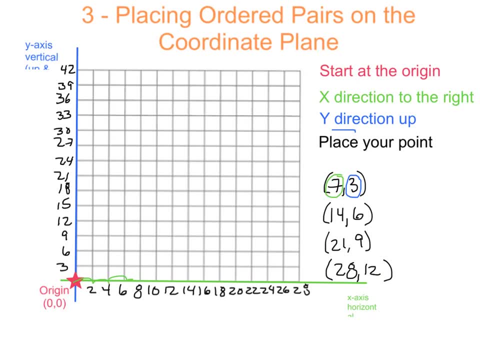 So we're going to go up 3.. So for here, we know that 3 is this first line, so then I'm going to go up 3.. And then we're going to place our point, which happens to be at the area where the 7 and the 3 cross. 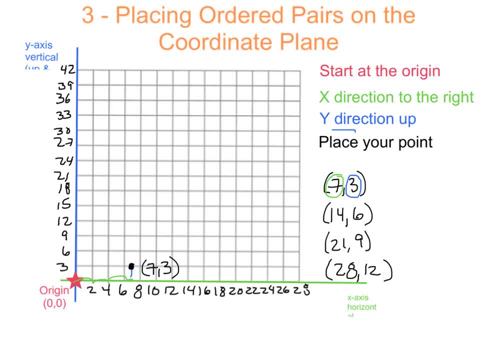 So that's our first point. So we're going to go up 3, and we're going to place our point, which is 7, 3.. Now let's see what all the rest of them will look like. Now I have my four other ordered pairs on our coordinate plane.